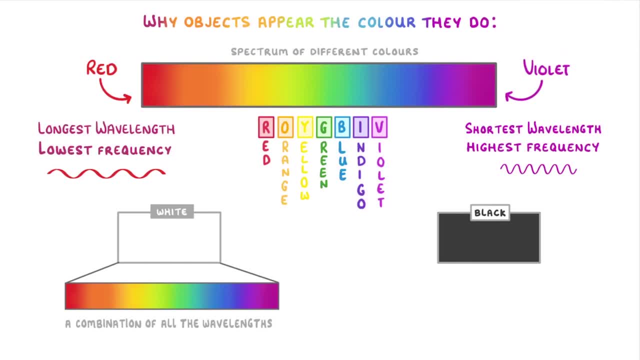 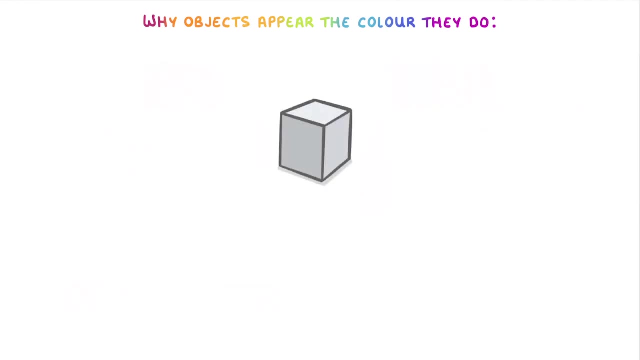 is a combination of all the wavelengths which together make white, and blackness is just an absence of light. So if there is no light, it will appear black. Now, which particular colour an object appears depends on two things: The wavelengths of 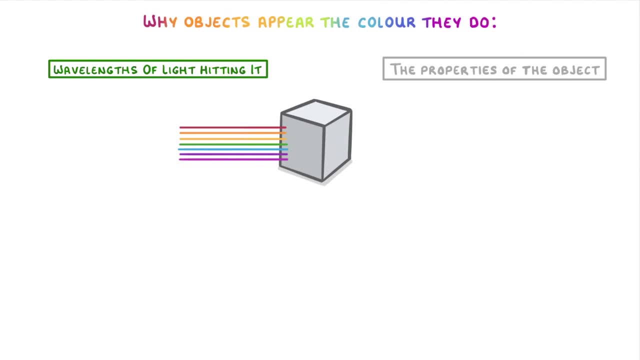 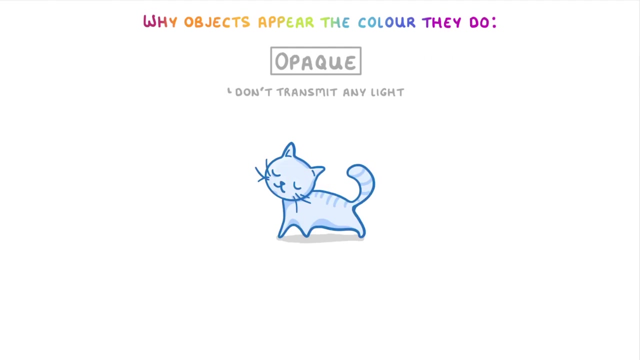 light that are hitting it and the properties of that particular object. Together, these will determine which light rays are absorbed, reflected or transmitted, and so determine how the object appears. Opaque objects are those that don't transmit any light, like a cat, This means that all 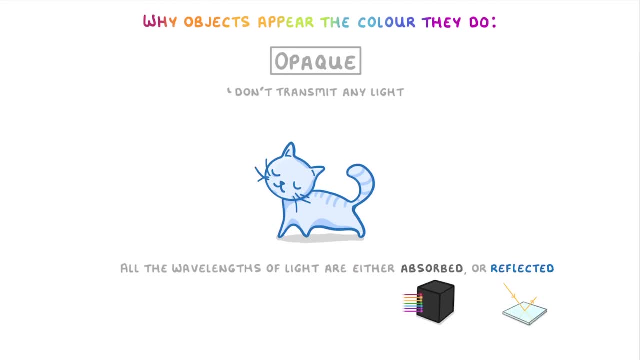 the wavelengths of light are either absorbed or reflected, and it's the reflected ones that determine the colour. So this cat appears blue because it's reflecting the blue wavelengths of light and absorbing all of the others. In some cases, though, an object might reflect 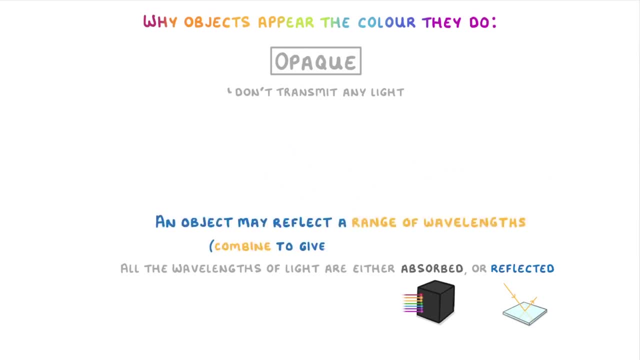 a range of wavelengths that together combine to give a particular colour. For example, this piece of cheese might appear yellow because it's reflecting yellow wavelengths, or because it's reflecting both red and green wavelengths, which combine to make yellow. Transparent and translucent objects, on the other hand, transmit lots of the light that 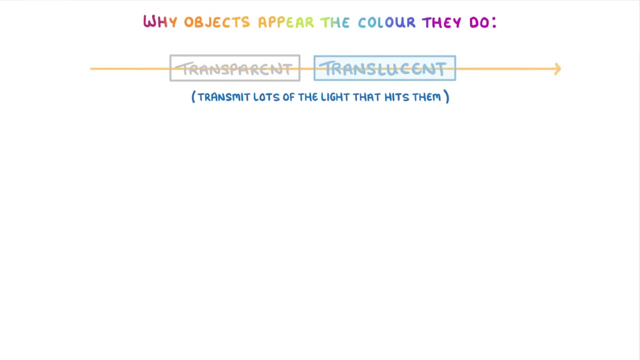 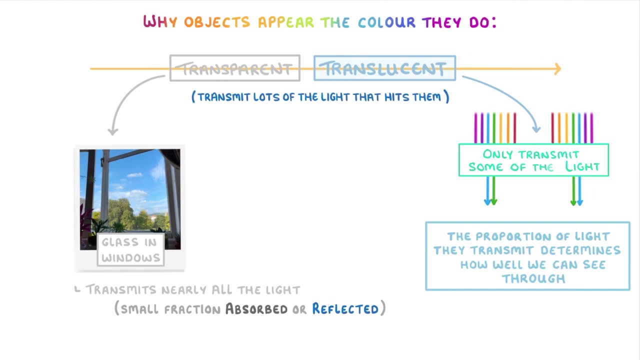 hits them, Which means that it passes straight through. For transparent objects, like the glass in windows, they're almost completely see-through because they transmit nearly all of the light, with only a small fraction being absorbed or reflected. Meanwhile, translucent objects only transmit some of the light and the proportion of light. 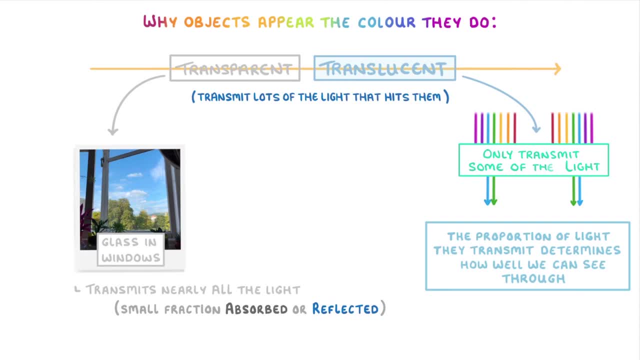 they transmit determines how well we can see through them. The colour of a translucent object is the colour of the light that hits it, and the colour of a transparent object, like a plastic bottle, is normally determined by which wavelengths are transmitted most. For example, this bottle appears green because the green wavelengths 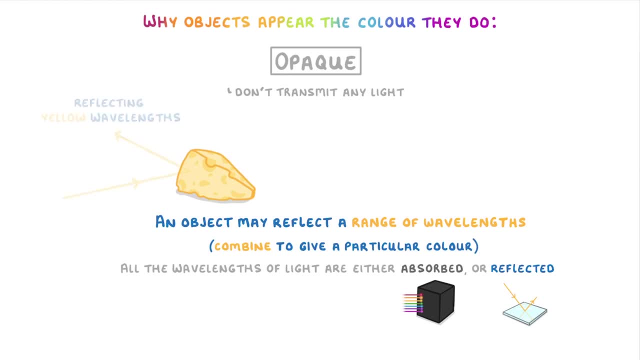 For example, this piece of cheese might appear yellow because it's reflecting yellow wavelengths, or because it's reflecting both red and green wavelengths, which combine to make yellow. Transparent and translucent objects, on the other hand, transmit lots of the light that hits them. 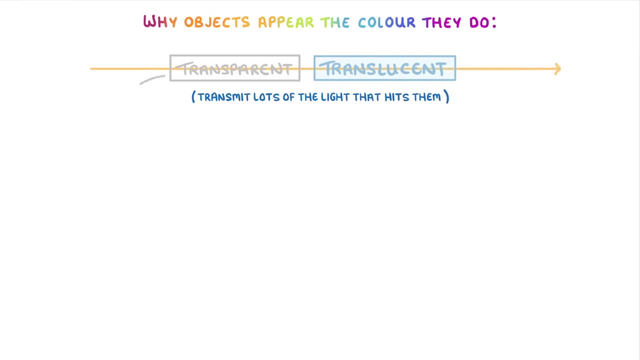 Which means that it passes strongly For transparent objects like the glass in windows. they're almost completely see-through because they transmit nearly all of the light with only a small fraction being absorbed or reflected. Meanwhile, translucent objects only transmit some of the light and the proportion of light. 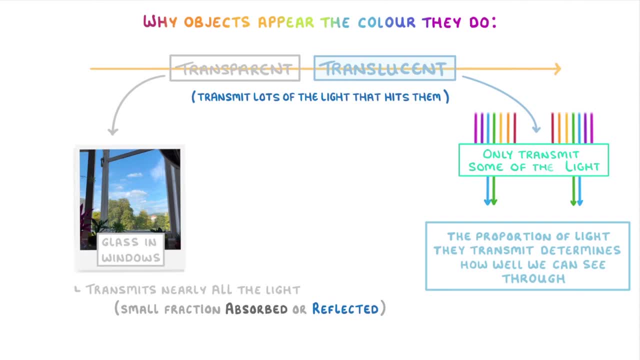 they transmit determines how well we can see through them. The colour of a translucent object, like a plastic object, is the same as the colour of a plastic bottle. It's normally determined by which wavelengths are transmitted most. For example, this bottle appears green because the green wavelengths are being transmitted. 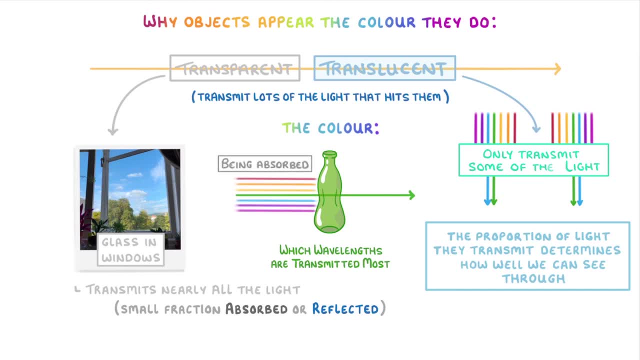 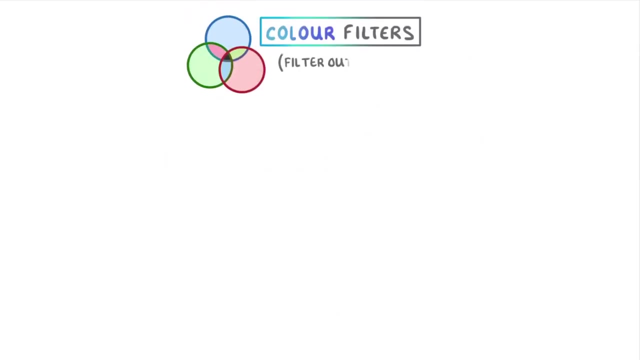 most, whereas the other wavelengths are being absorbed and so aren't reaching our eye, like the green wavelengths are. The last thing we need to look at are colour filters, which are used to filter out particular colours, such as colour filters. They work by only transmitting certain wavelengths of light, while absorbing the rest. 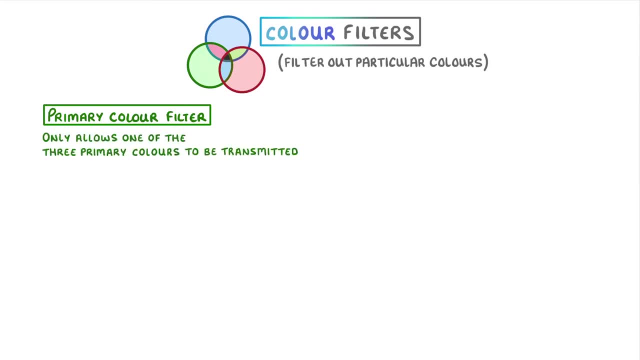 A primary colour filter is one that only allows one of the three primary colours to be transmitted. so red, green or blue, For example. if we put white light, which, remember, contains all the different wavelengths, we can only transmit one of the three primary colours. 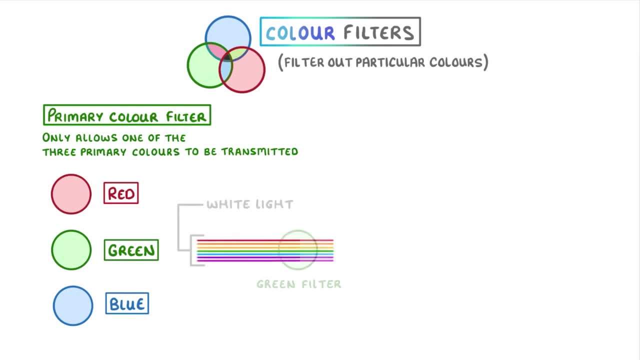 This means that if we put white light, we can only transmit one of the three primary colours, Just like in the picture. if we put two different wavelengths of light through a green filter, then only the green wavelength would get through. So if we looked at white paper through this filter, then it would appear green because 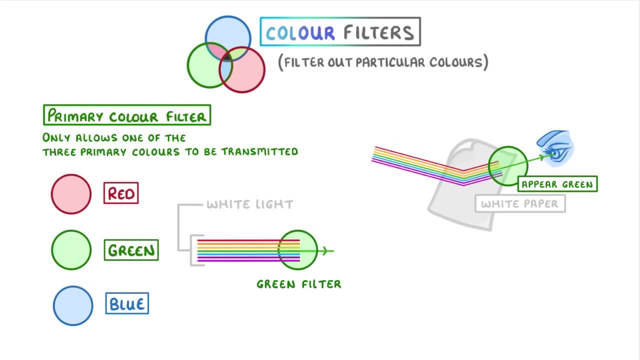 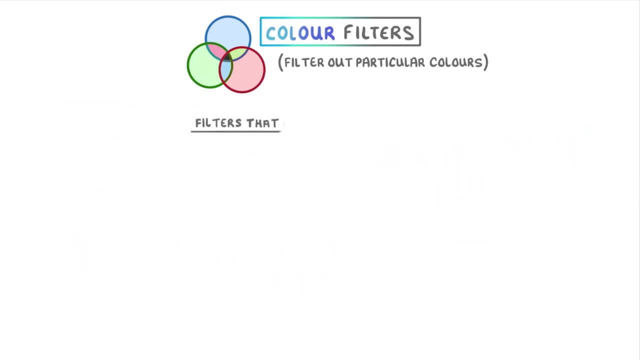 only the reflected green waves would make it through, Whereas if we looked at a blue object, which must be reflecting only blue light, through a green filter, then it would appear black because the filter would block the blue light from passing through, so no light would be reflected into your eye. Filters that aren't for primary colours. 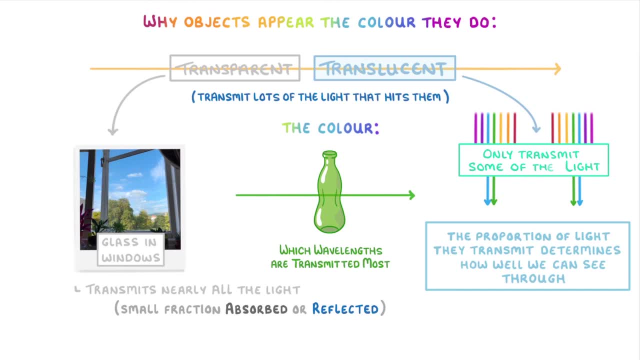 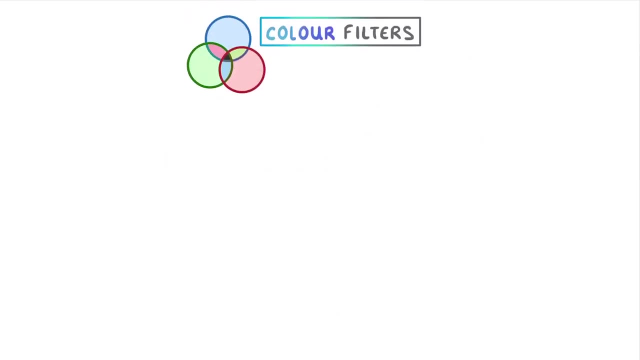 are being transmitted most, whereas the other wavelengths are being absorbed and so aren't reaching our eye, like the green wavelengths are. The last thing we need to look at are colour filters, which are used to filter out light, to filter out particular colours, so that only certain wavelengths can pass through. 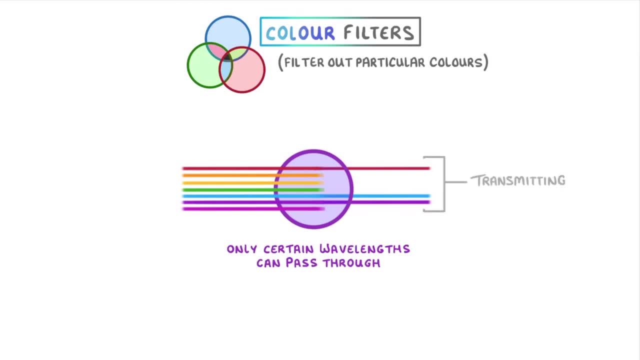 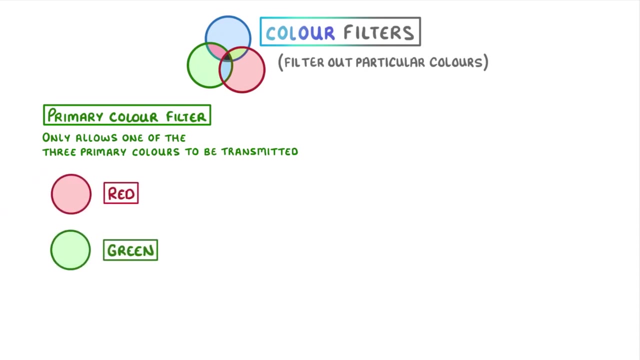 They work by only transmitting certain wavelengths of light while absorbing the rest. A primary colour filter is one that only allows one of the three primary colours to be transmitted. so red, green or blue, For example, if we put white light- which, remember, contains a lot of light, and we're 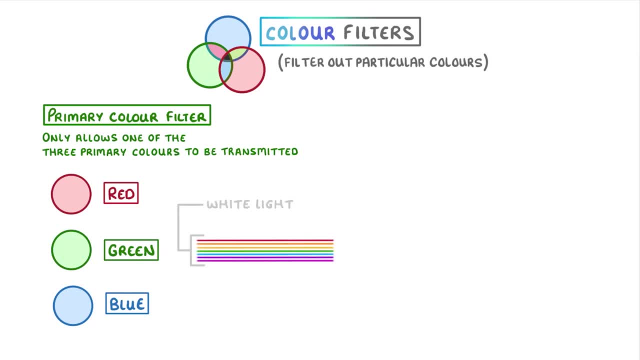 only transmitting one of the three primary colours. we're only transmitting one of the three primary colours. If we put green light, which contains all the different wavelengths of light, through a green filter, then only the green wavelength would get through. So if we looked at white paper through this filter, then it would appear green, because 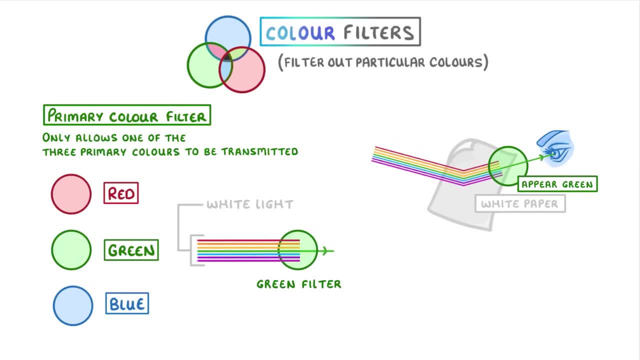 only the reflected green waves would make it through, Whereas if we looked at a blue object, which must be reflecting only blue light, through a green filter, then it would appear black, because the filter would block the blue light from passing through, and so no light would be reflected into your eye. 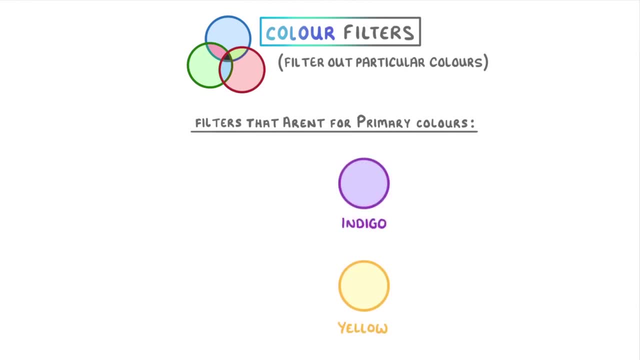 Filters that aren't for primary colours, like yellow or indigo. filters let through both the wavelengths of light that are the same colour as the filter and also wavelengths of the primary colours that can be added together to make that colour. For example, yellow filters will let through yellow light but also let through red and 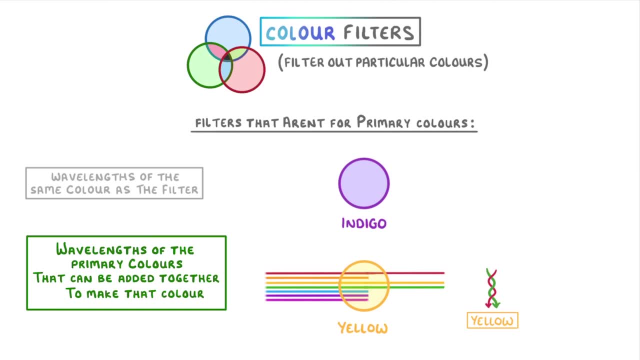 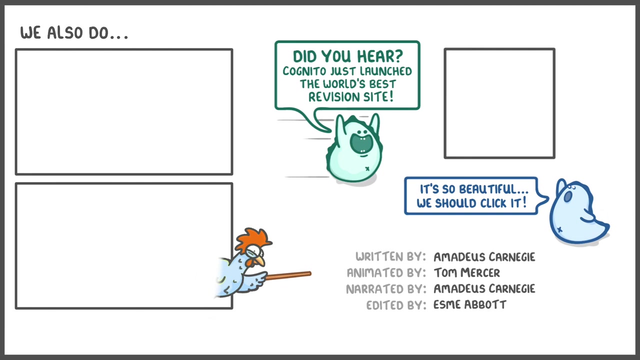 green, because red and green combine to make yellow. Meanwhile, indigo filters will let through indigo wavelengths, but also let through blue and red, as blue and red light combine to make indigo. Anyway, that's everything for this video today, so hope that all made sense and we'll see. 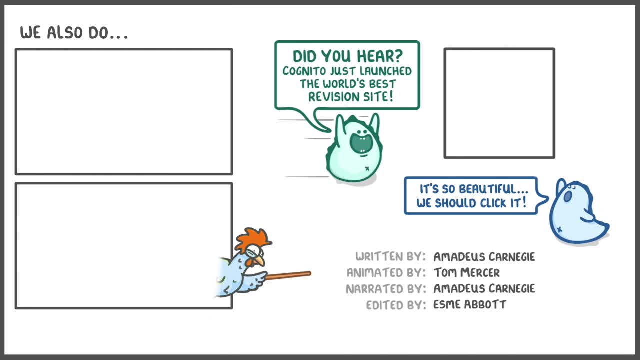 you again soon. Subtitles by the Amaraorg community.